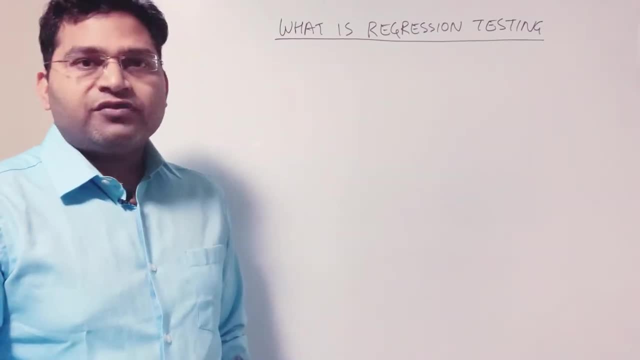 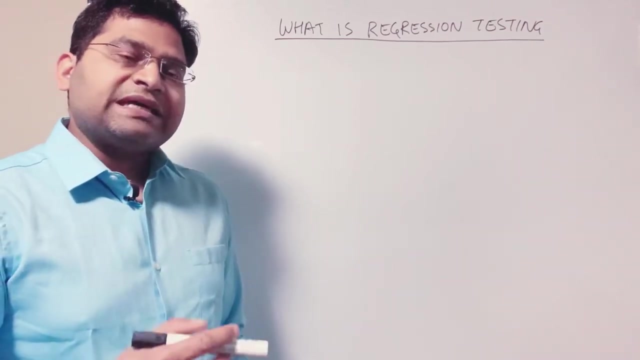 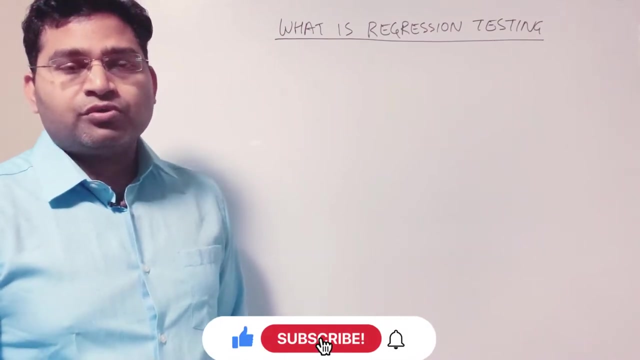 that the existing functionality of the software or application works as expected if there is any new code introduced or new defect fix has been done or any new functionality added in the application. So please note that regression testing is, you know, different from retesting. So retesting is sort of you know. 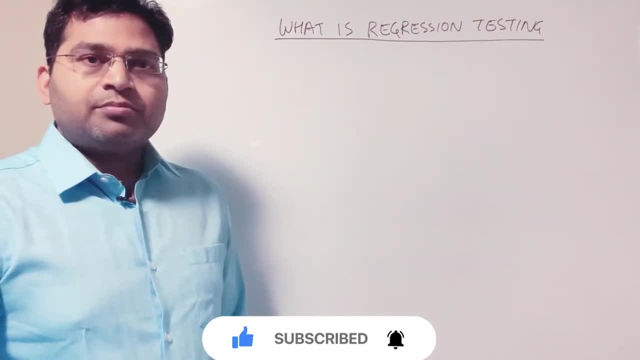 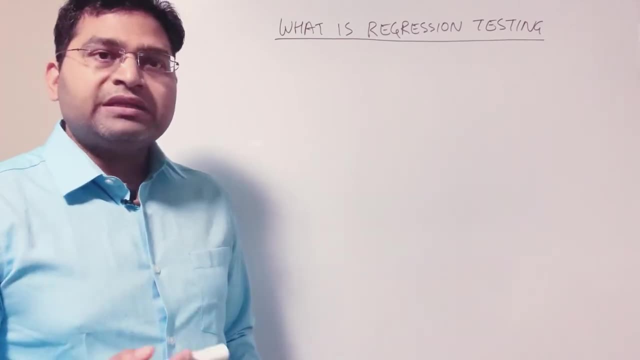 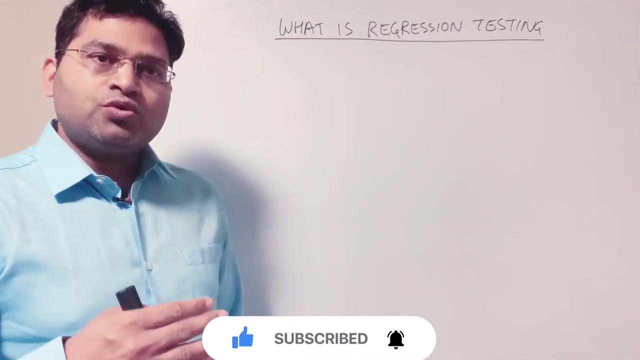 you can say it's a part of regression testing, but there is a very fine difference between regression testing and retesting, right? So you need to understand from interview point of view, that regression testing is not same as retesting. But in regression testing you do some retesting. 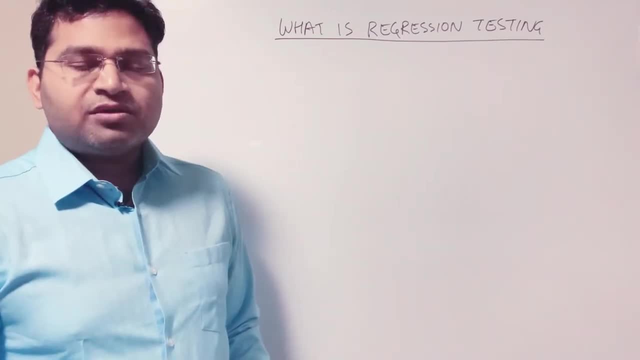 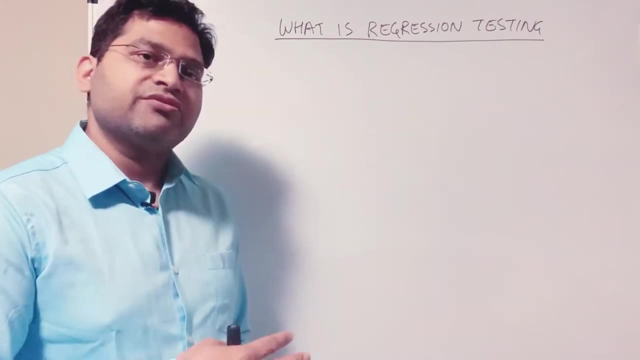 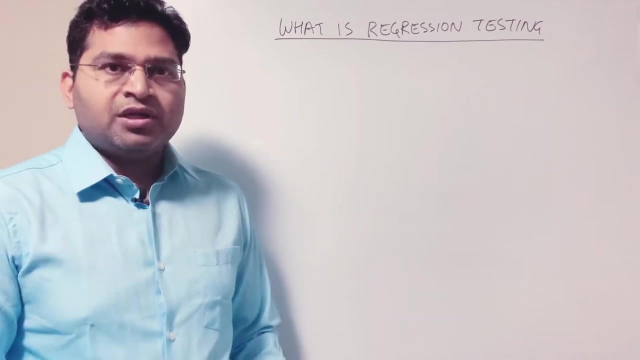 So you can say there are, you know, some retesting, or the test case that you execute as part of regression testing are the test cases that you are actually retesting. But the definition and the purpose of regression testing and retesting is completely different. So let's first understand what exactly regression testing is and when you do. 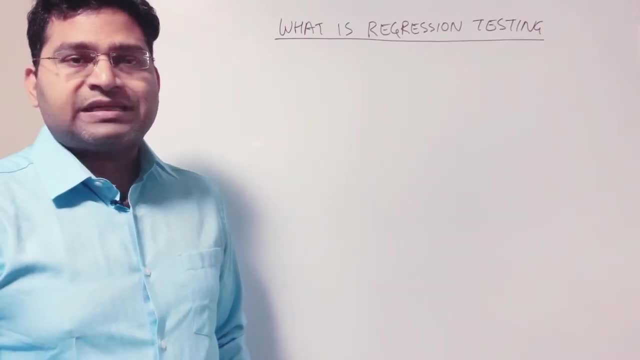 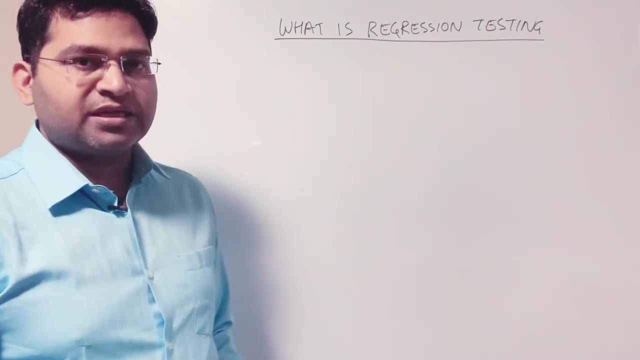 it, how you do it, what are the different strategies or techniques that you use to do regression testing? Now let me take an example to explain you exactly what regression testing is. So, in terms of definition, regression testing is a test case that you execute as part of regression testing. 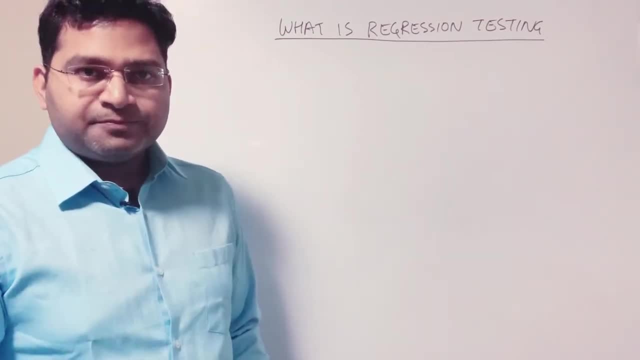 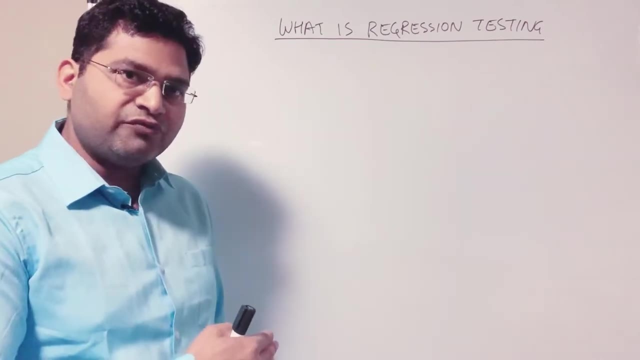 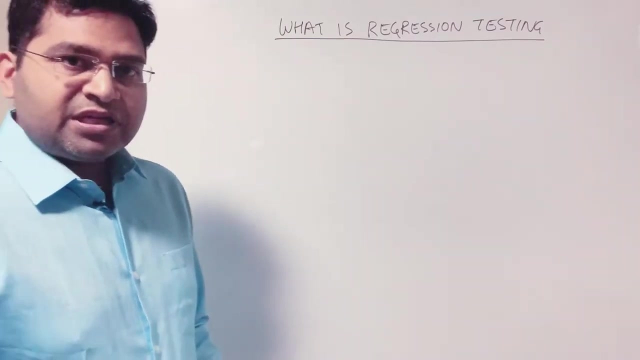 We know that any you know testing that you perform if there is any bug fix or code changes or new functionality addition into the software that you know set of test cases that you execute, is the regression testing. Now say, for example, if I take an example of the e-commerce website: 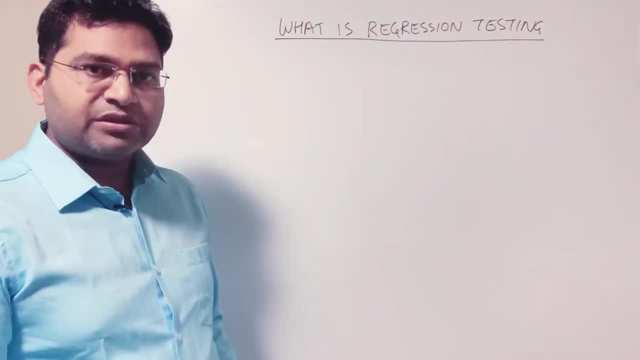 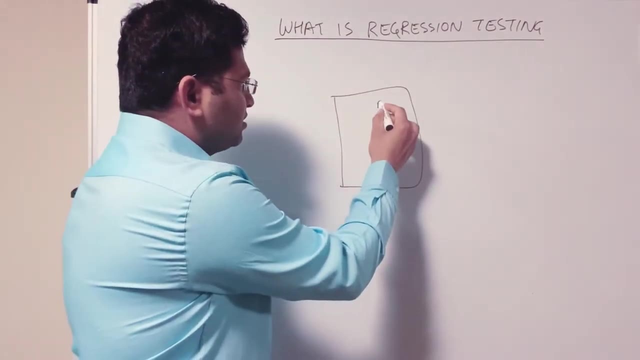 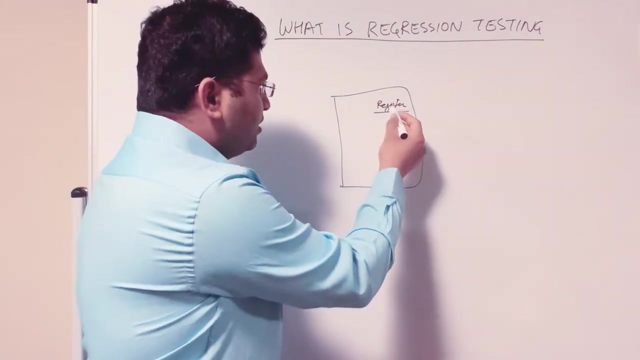 so e-commerce website will have the register functionality right. So that is the example that we have been taking till now. Now in the registration page, say, for example, there is a register link and once the user clicks on a register link he has the option to register. 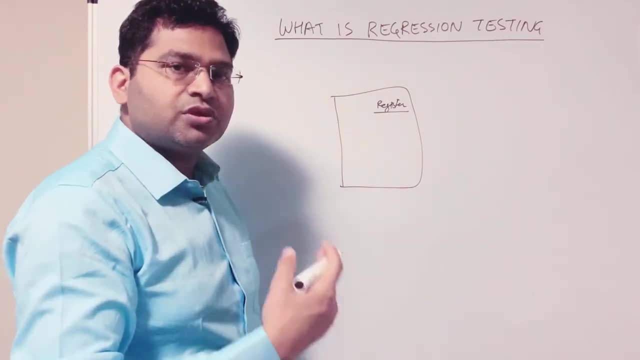 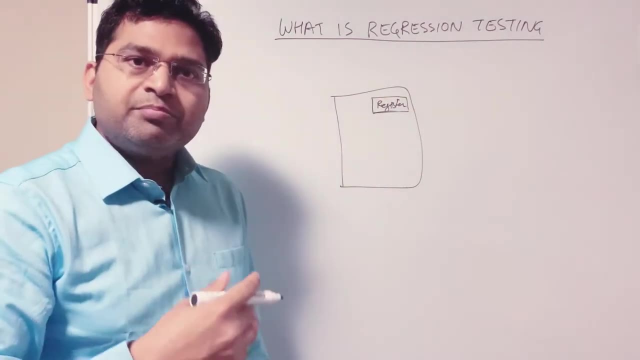 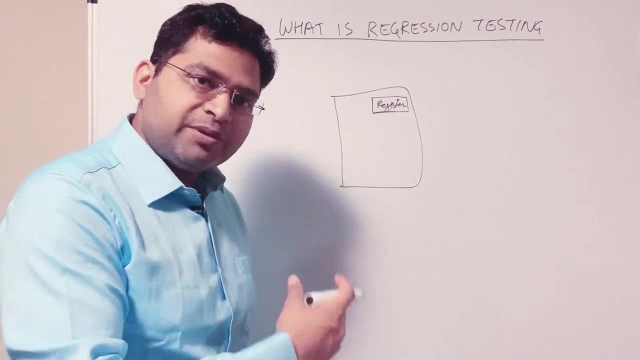 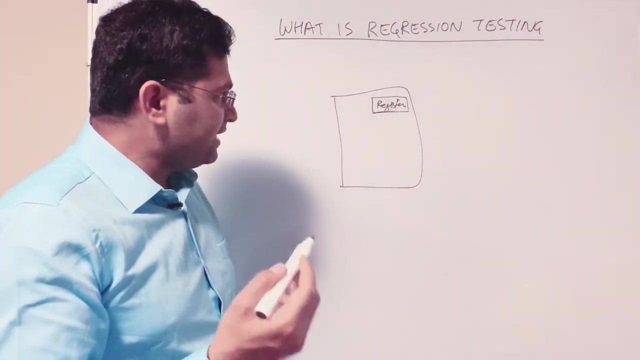 using email, using Facebook account, using Google account and other social media accounts, right? So in the register module, there are many different options, basically, or different implementation to register a user on the particular website or an e-commerce website. Now, when the user registers on an e-commerce website, then in that particular case, if there, 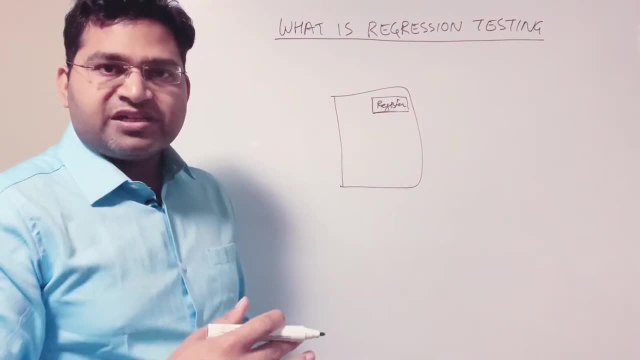 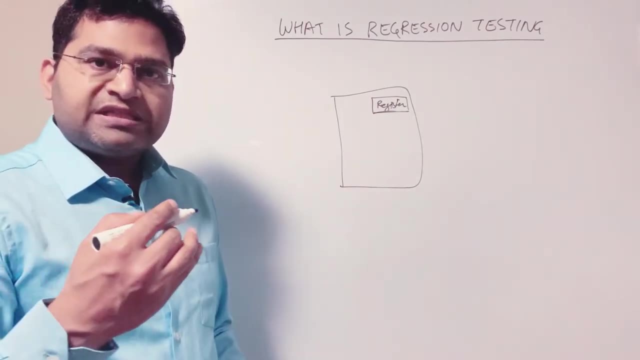 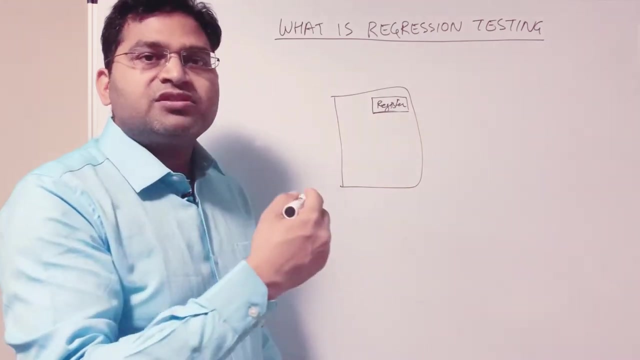 is any change? say, for example, you are testing the registration functionality and during the testing of the registration functionality with the Facebook registration or registration using Facebook login ID, the registration fails or registration is not successful. So that is the defect that you found during the functional testing. 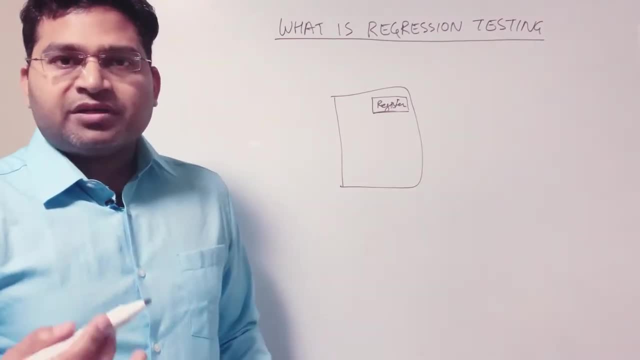 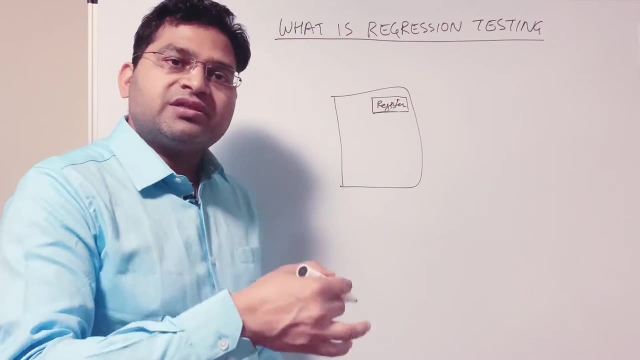 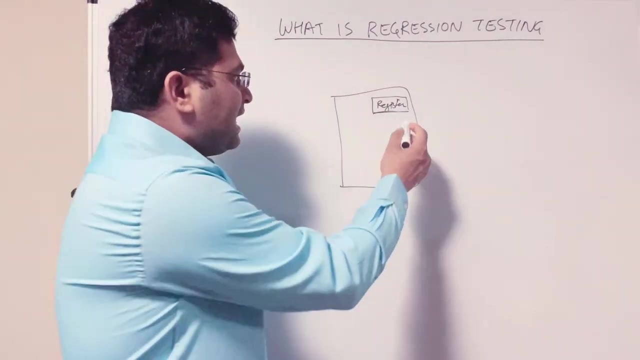 Now, when the developer is fixing that particular defect, then in that case that fix could impact other registration functionality as well in the application right. So when the defect of registration got fixed, then in that case what you need to do is 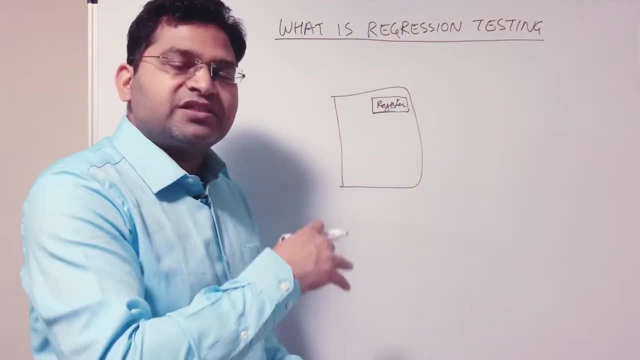 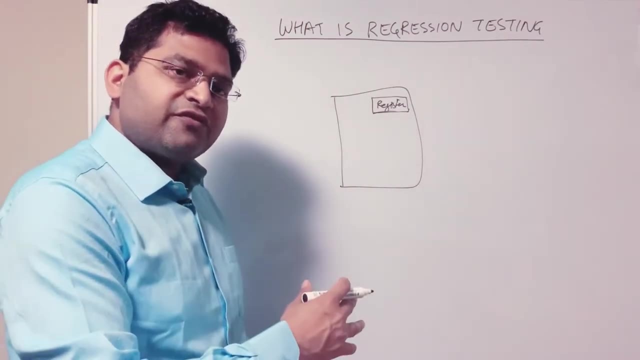 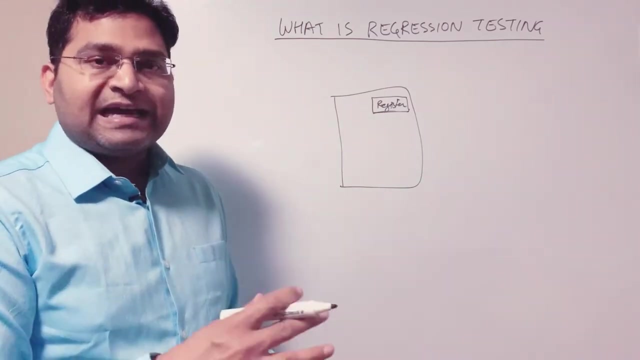 you need to basically verify that other registration functionality is also working as expected. Now, when you are verifying the other registration functionality or you are testing the registration functionality using email using Google account as part of the defect fix that was fixed for the Facebook account, 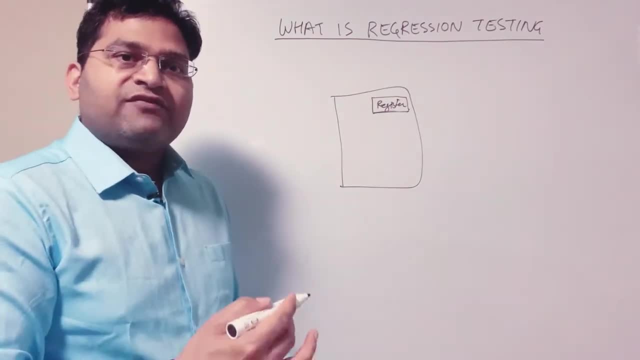 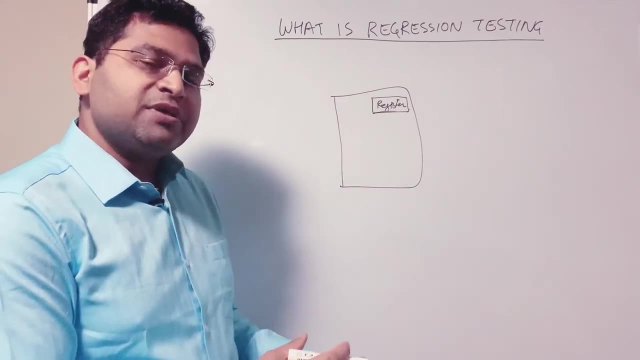 then those test cases that you'd execute as part of this defect fix are known as regression test cases, right, Or regression testing. Now, regression testing is not limited only to that set of test cases. It could be a complete set of regression test cases. 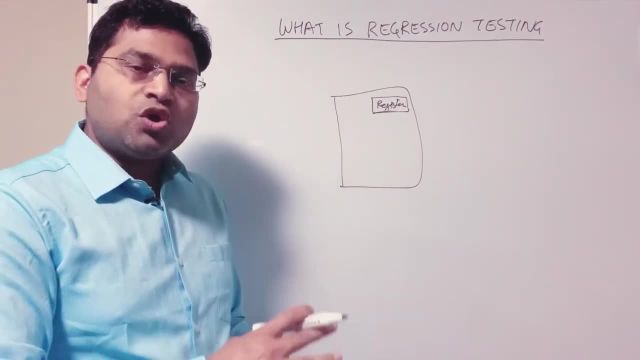 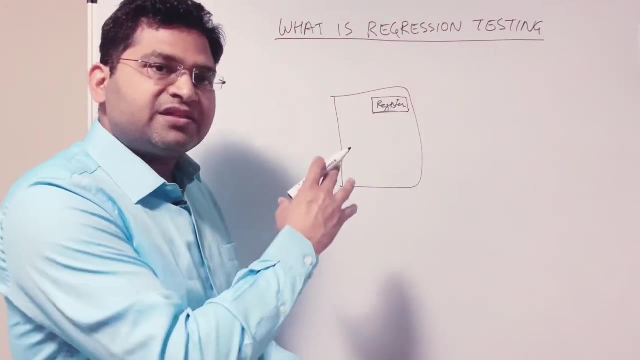 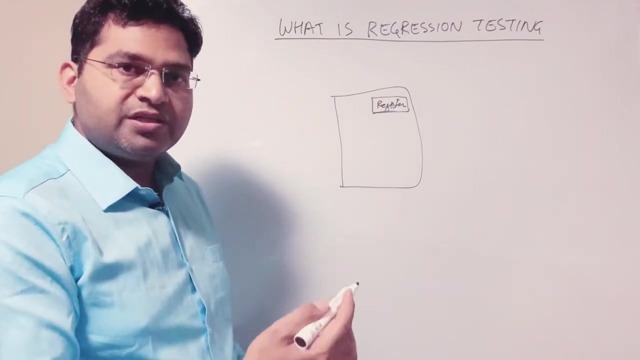 In this particular case, if say, for example, you want you can test the overall critical functionality of the whole e-commerce website because there has been a fix that is done within the application. So there are different techniques that can be chosen to do the regression testing. 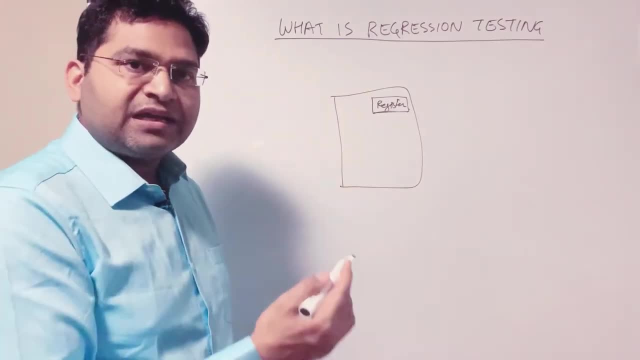 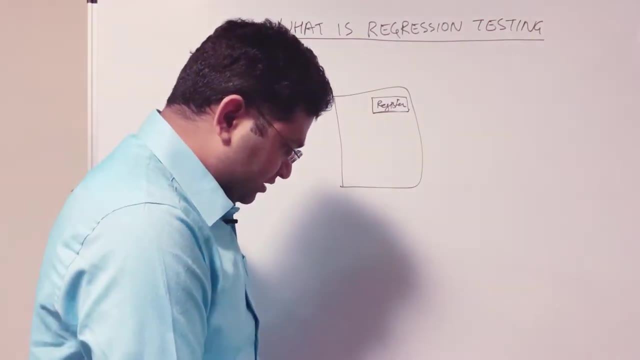 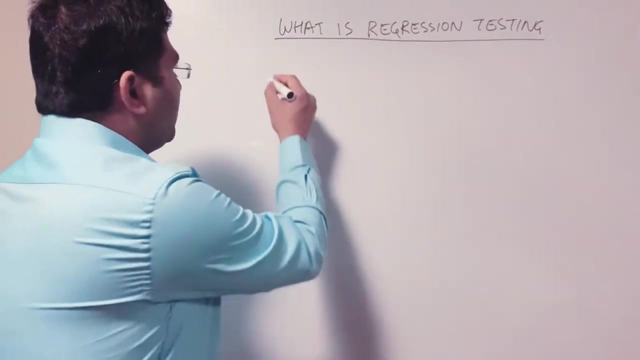 So this is a brief introduction and what exactly regression testing is and when you should do regression testing. Now let me first understand. you know what all scenarios could be there when you can perform regression testing. right, So let me say when you. 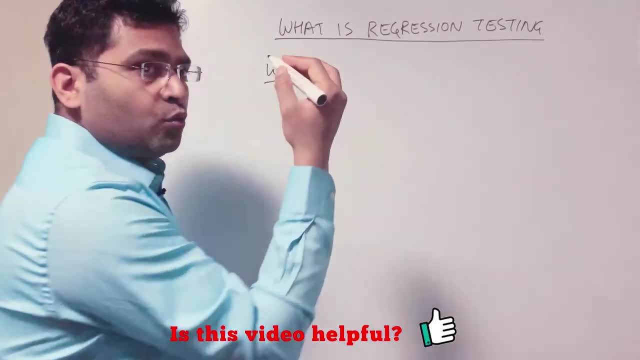 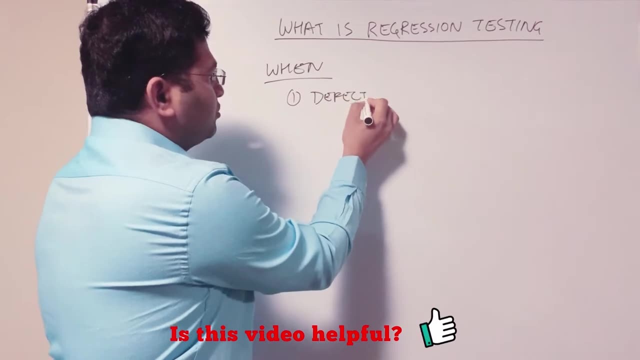 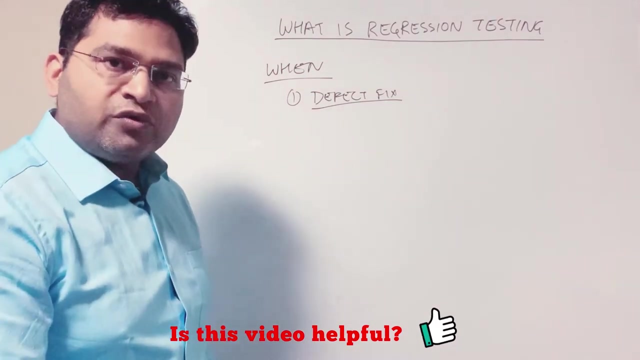 can do regression testing. So if I talk about when, so the first example that we took is when the defect fix happened right. So in the case of defect fix, So when we say defect fix, defect fix will be done when there is a code fix right. So if there is any defect there could be, you know. 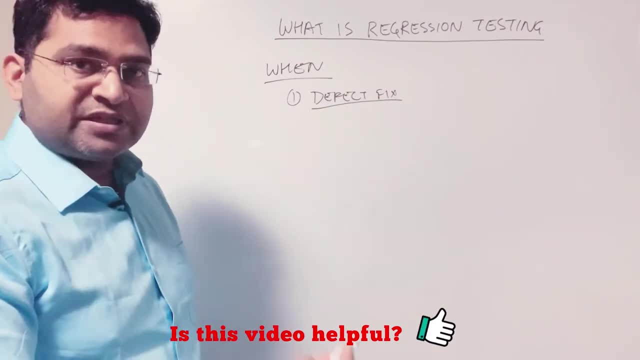 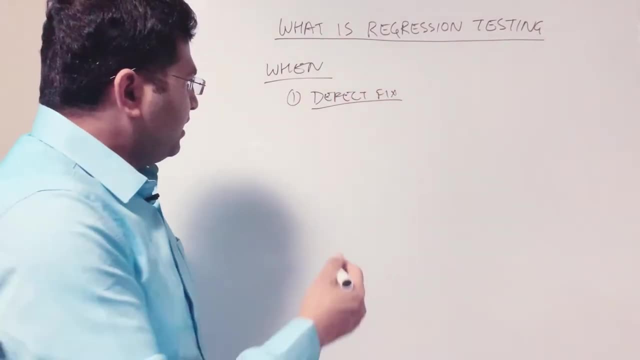 a code fix or there could be configuration changes that could fix that defect right. So in case of defect fix, there will be the need of the regression testing, okay. And the second option could be new functionality- right, So new functionality added. 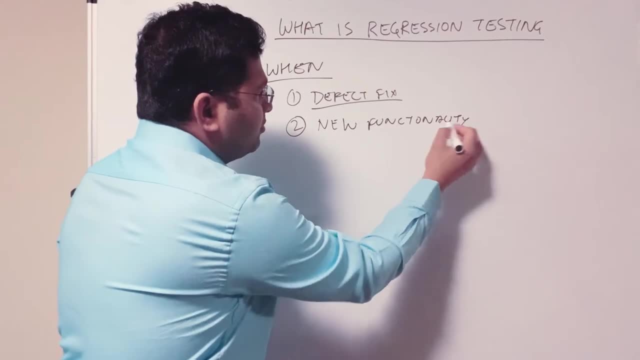 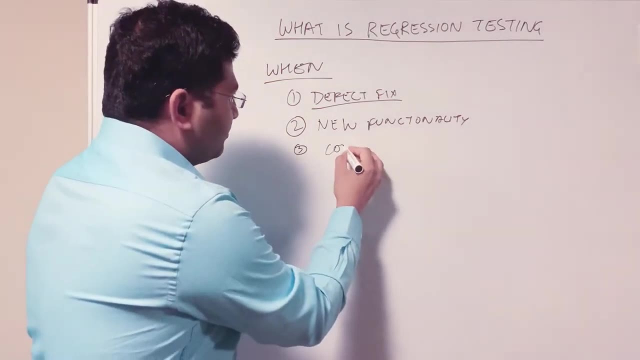 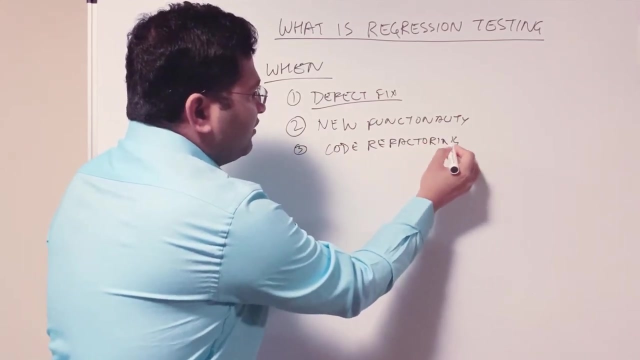 So new functionality or feature being added into the application. So that could be the second case. Third case could be code refactoring- right, So code refactoring, wherein developers or the development or development team refactors the existing code to improve the performance, or 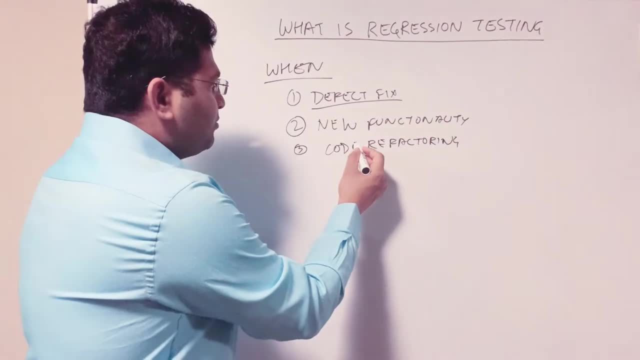 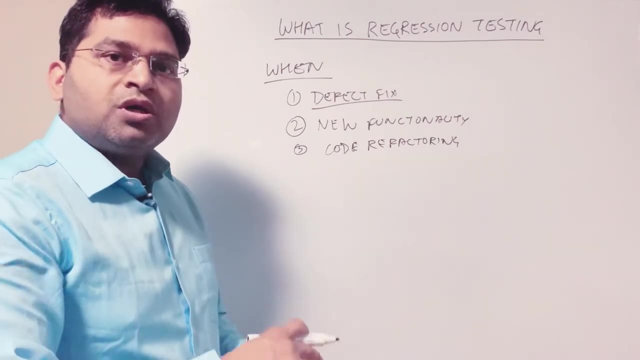 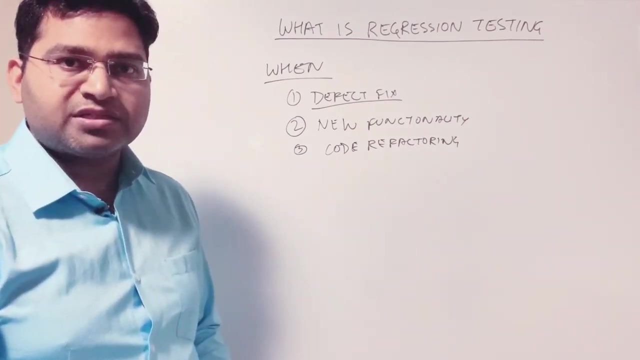 improve the maintainability of the code, Then in that particular case the overall structure or the code is being refactored. In that case you need to pick a set of test cases that are critical for that application and are basic to that particular application and ensure that the 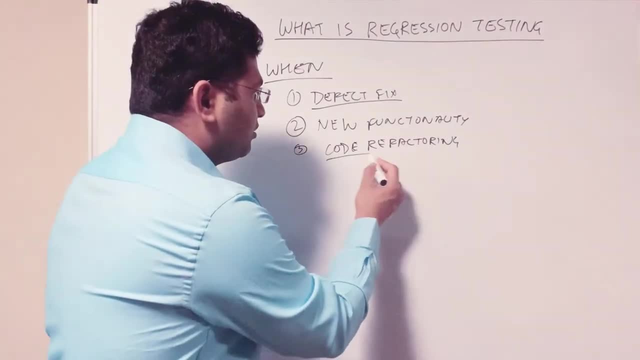 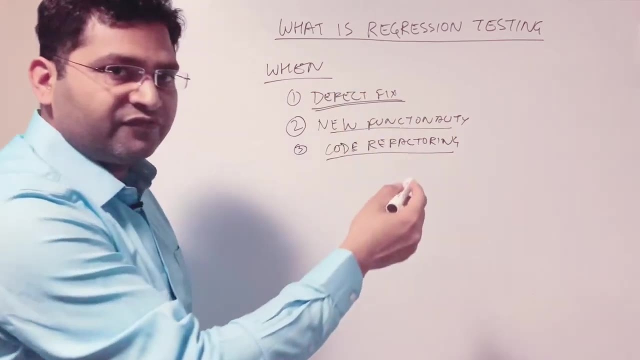 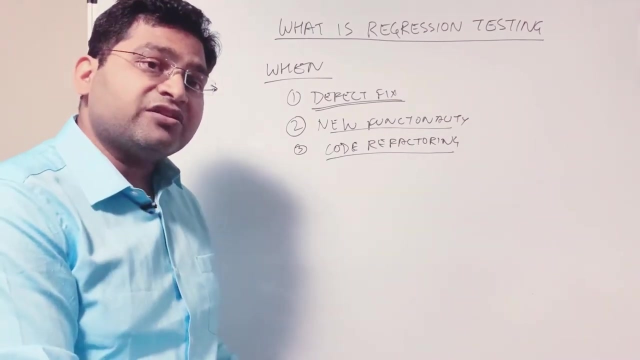 application functionality has not been impacted because of code refactoring or because of adding the new functionality or because of having the defect fix in the application. So any verification that you do to ensure that the existing functionality of the application because of defect fix, new functionality, code refactoring- there could be any number. 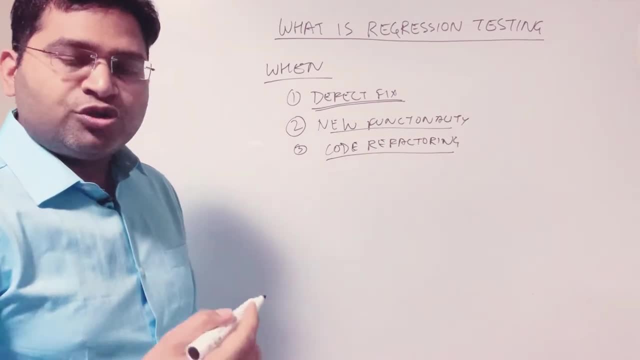 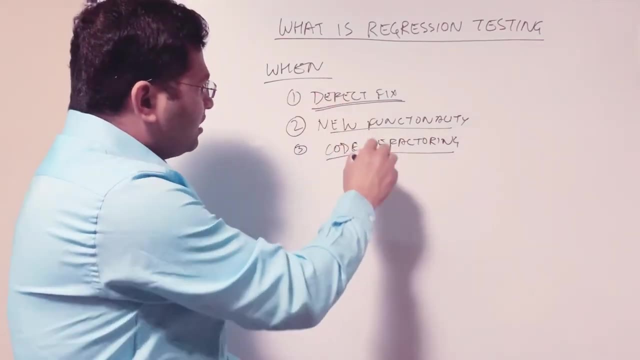 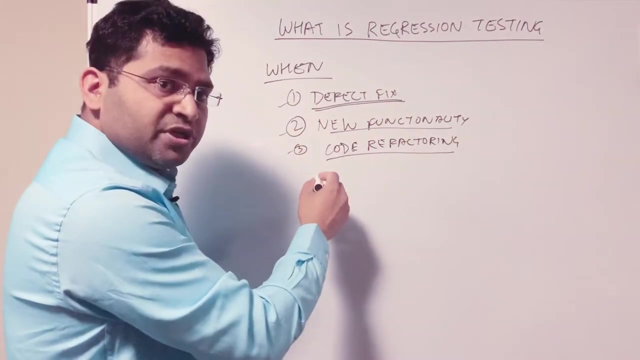 of other factors as well and ensure that the existing functionality of the application works as expected. then that is regression testing, And these are some of the places when you do regression testing There could be. this is not the comprehensive list. there could be many more factors when 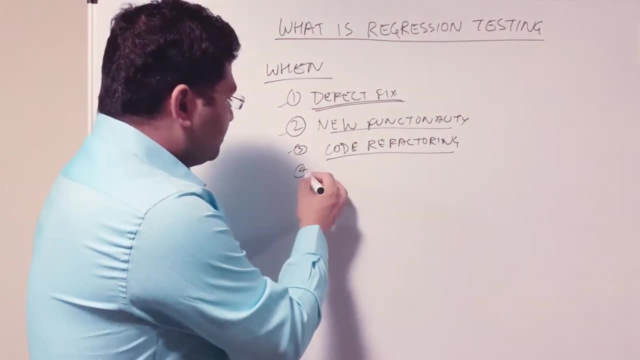 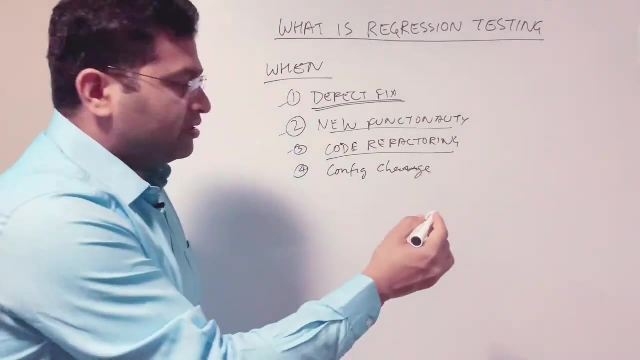 you choose to do regression testing. Other I can think of is say, for example, configuration changes, so config changes. So if there are any config changes in the application, then in that case as well you do regression testing. So this is when part of the configuration changes. 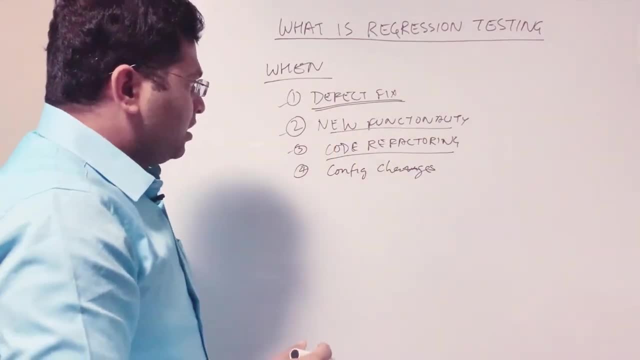 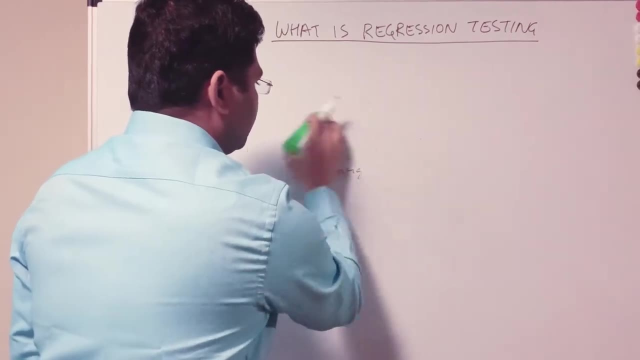 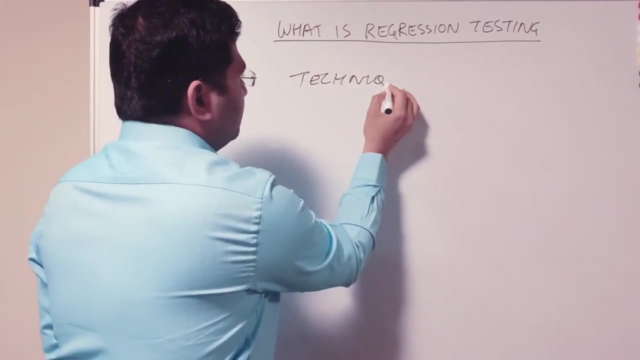 This is the part of the regression testing. So when you do the regression testing, Now, if I talk about the techniques of the regression testing, so let me say techniques, let me rub this, and in the techniques, so in the techniques of regression testing, what 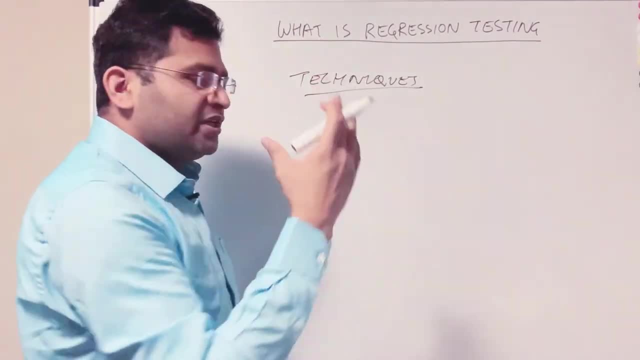 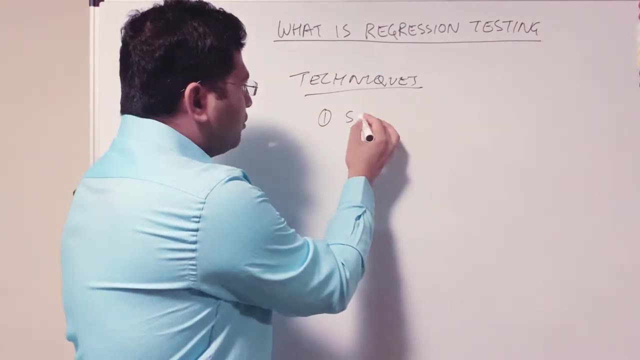 you can do is say, for example, there is a defect fix that we have seen in the e-commerce portal. So in the techniques you can. So the first technique will be: you can select all the test cases. so you can select all the test cases, that existing test cases for the application. 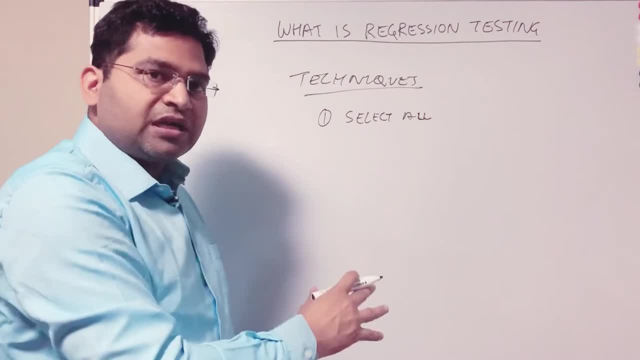 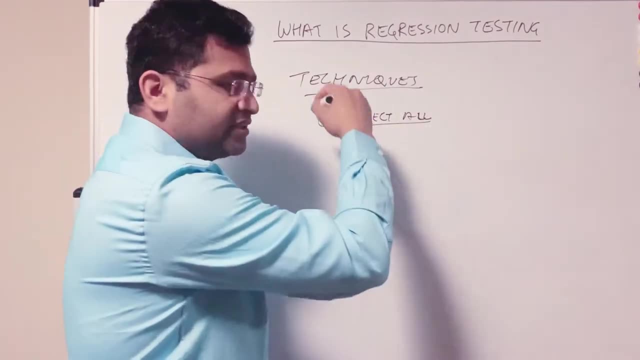 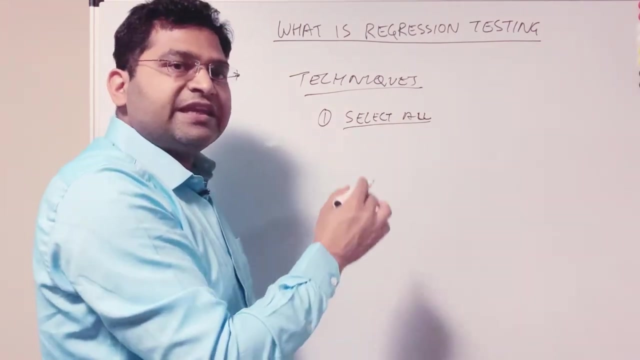 So in the e-commerce portal, whatever test cases you have written till now- say, for example, what are functionalities have been implemented- you can select all the test cases and execute all those test cases. So that could be one of the technique or approach to do the regression testing in case of any. 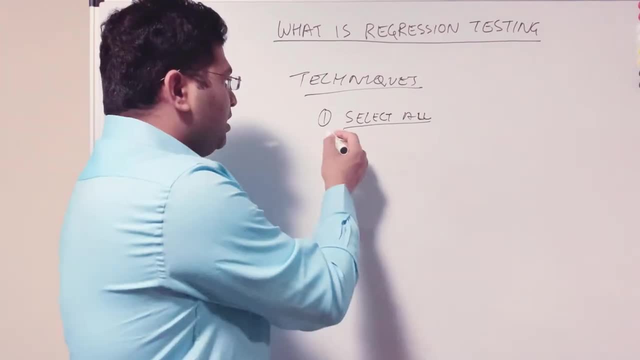 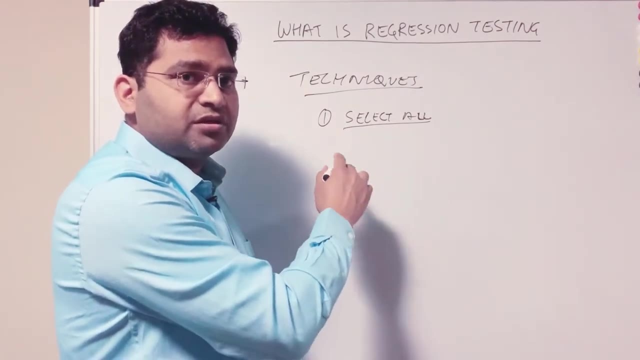 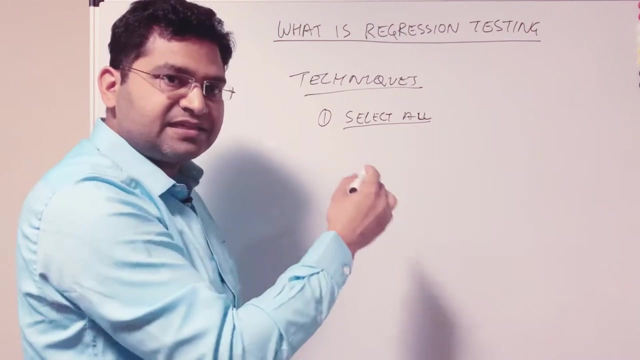 fix or any new functionality being added, Okay, But this is, this is very highly, you know, unlikely unless you are having a hundred percent automated regression test suite, because it will require a lot of manual testing effort to do the- you know- complete regression test after each of the defect fix. because you 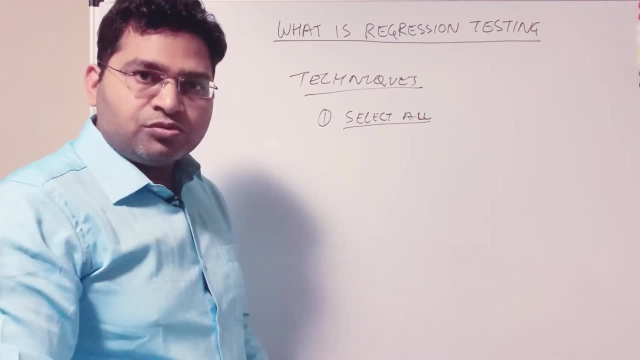 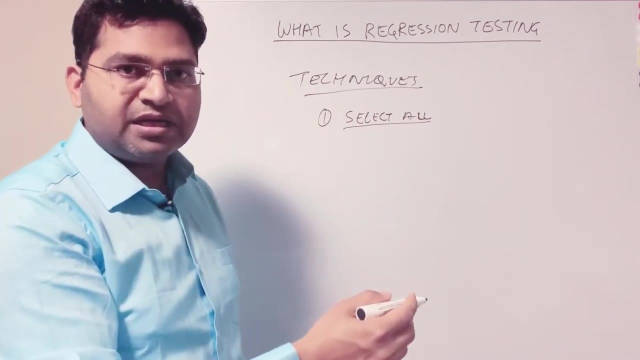 have to re-execute. So, for example, till release two you have written a hundred test cases. Then with every defect fix you have to basically re-execute those hundred test cases, right? Or with any new functionality being added. Okay. 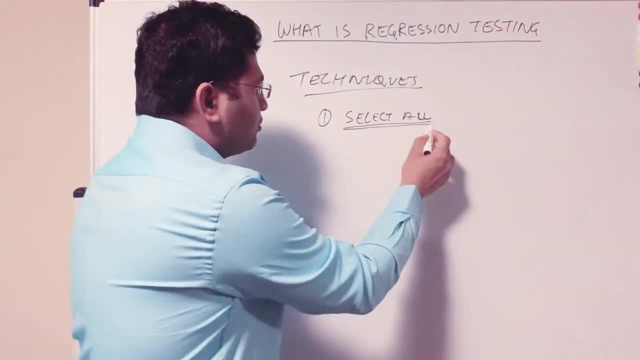 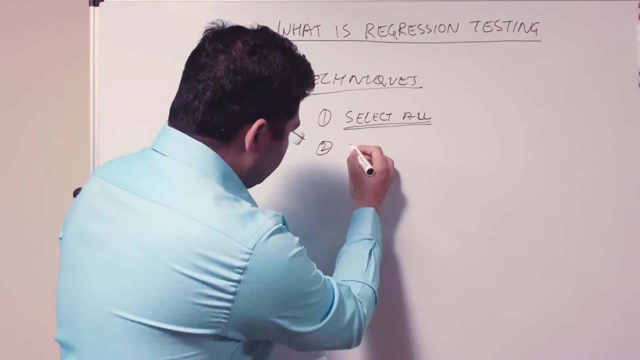 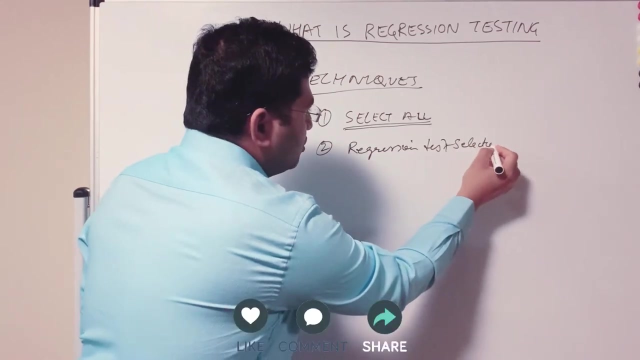 So you have to re-execute those hundred test cases if you do select all, or you select all the test cases. The second technique you can use is basically, you know, regression test selection, Okay, So in this case what you do is you basically see what area of the application has been. 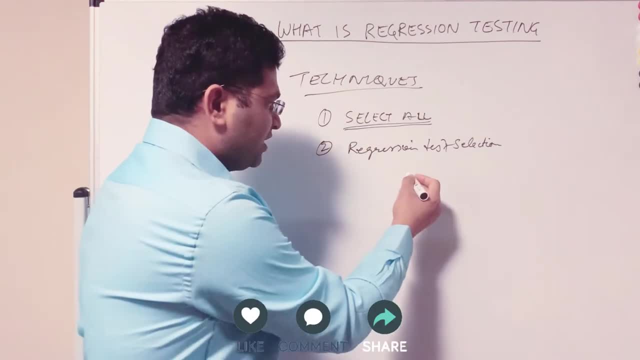 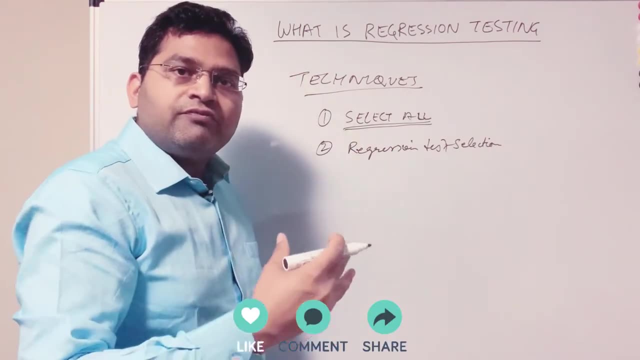 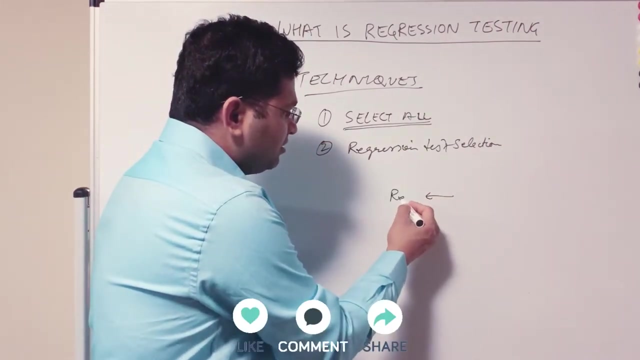 changed Now in this in. in the previous example we have seen the registration functionality. So in the registration functionality only the registration with Facebook was failing. Say, for example, right now that uh, fix has been done in the register. 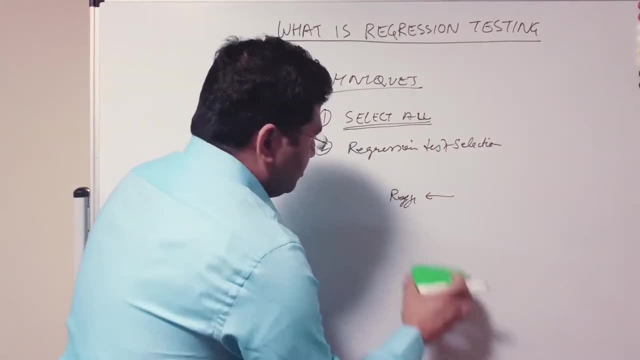 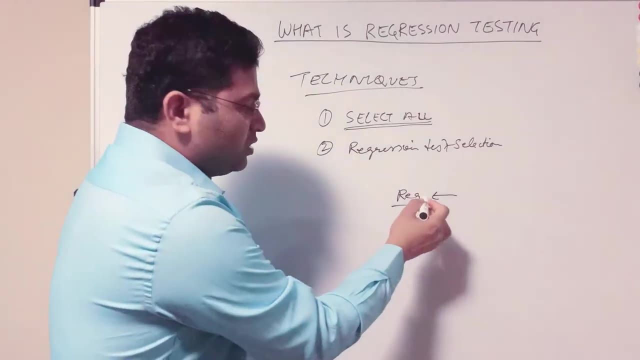 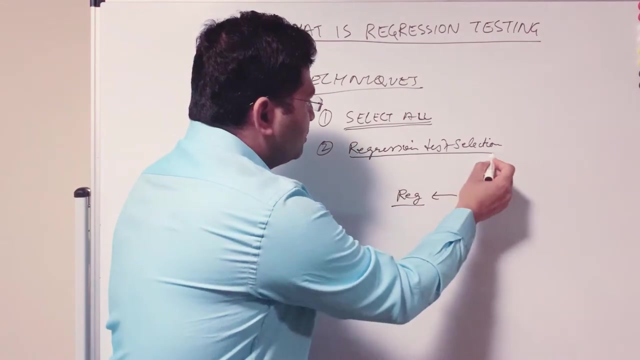 Okay So in the registration- pardon my handwriting, just uh, let me change it. Okay So in the registration, only the Facebook registration. uh, defect has been fixed, fixed. So what you can do is Yeah, Yeah. 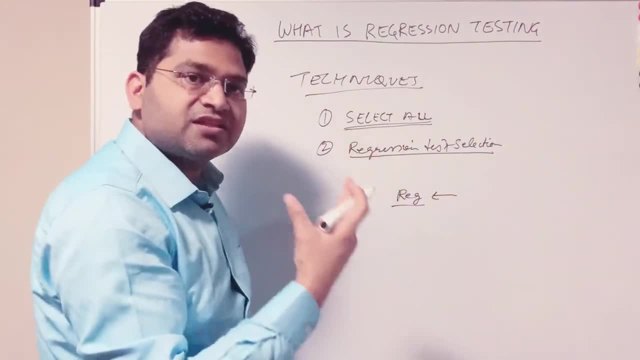 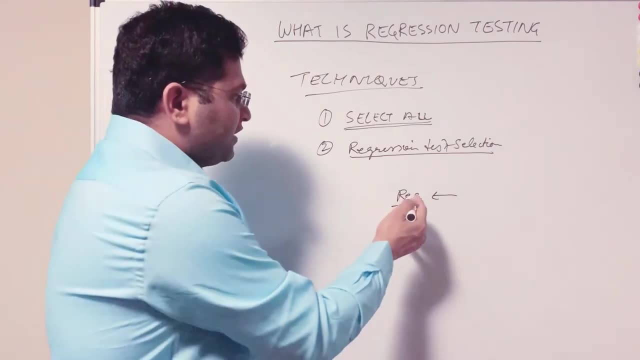 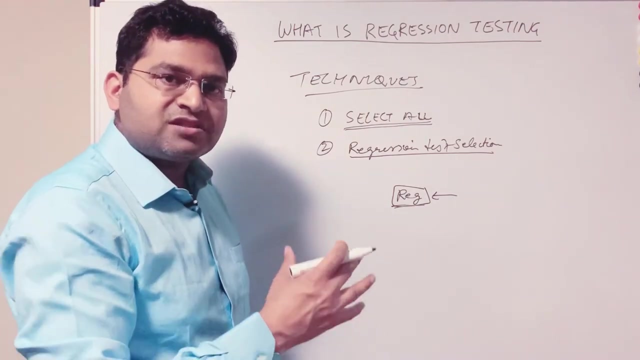 So in this particular technique. so what you do is you, you select the test cases that you want to execute or basically, you analyze the modules that could be impacted because of that particular fix. So now we see registration functionality. uh, is you know related? uh, so we'll test. 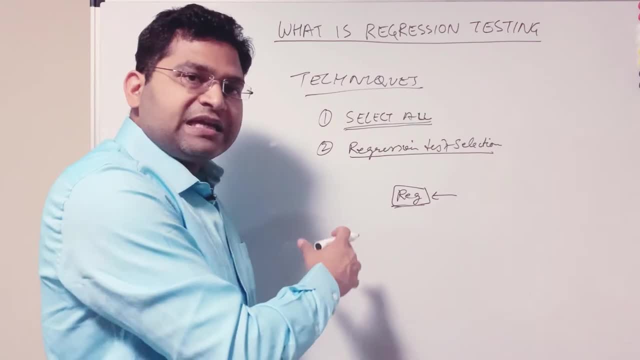 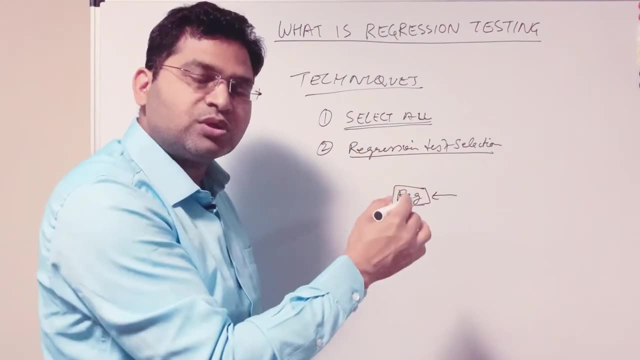 all the registration test cases with different, you know, social media account and email account, And we'll also test the login functionality along with that. Right, So you can have a subset of test cases. You can select the subset of test cases. 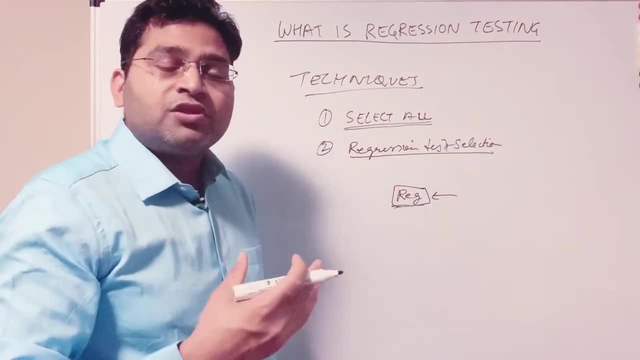 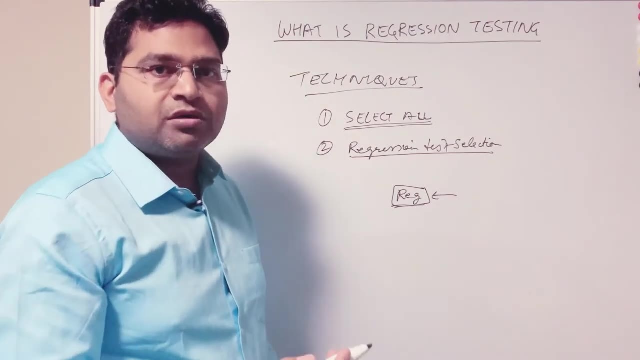 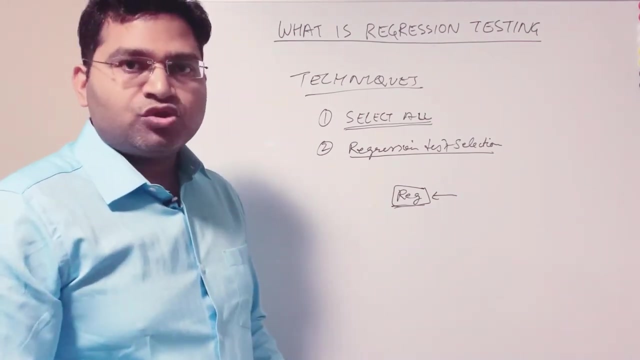 Uh based on your uh analysis of the module that has been changed or updated by the developer and developers. If you talk to developers, they'll help you out uh about the impact or the changes that they have done in the code, which will help you to analyze which test cases you need to. 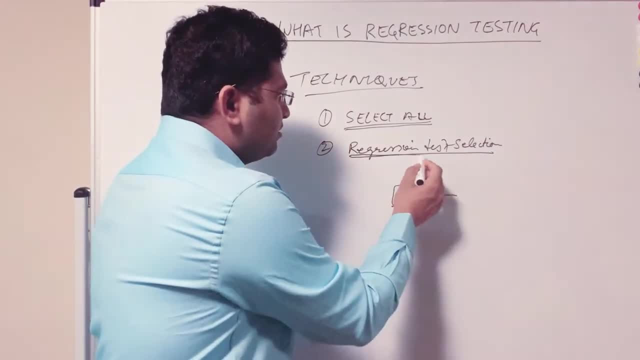 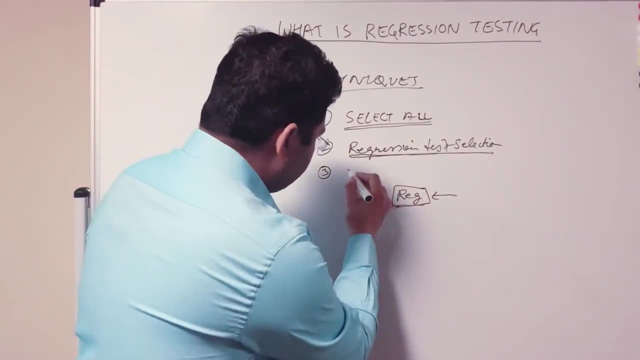 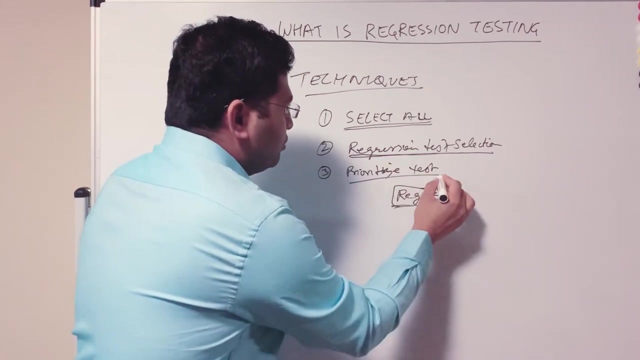 basically re-execute. when you, when you select uh the test selection for the regression, The third approach will be: uh, basically, you prioritize the test cases, right, So prioritize. So, in the prioritize uh test cases, what you do is you prioritize the critical test. 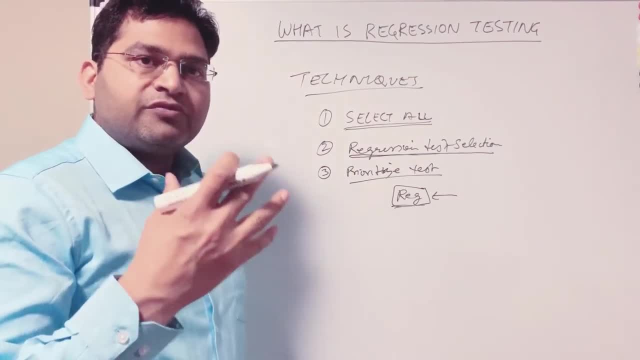 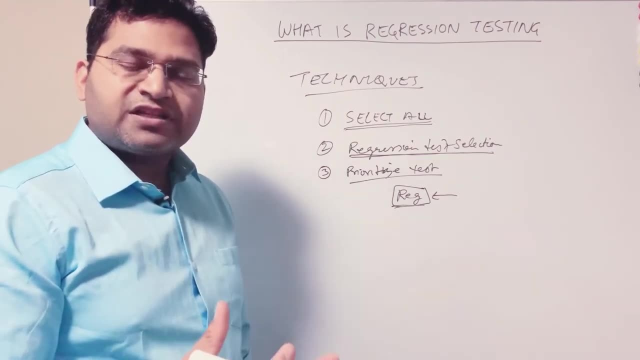 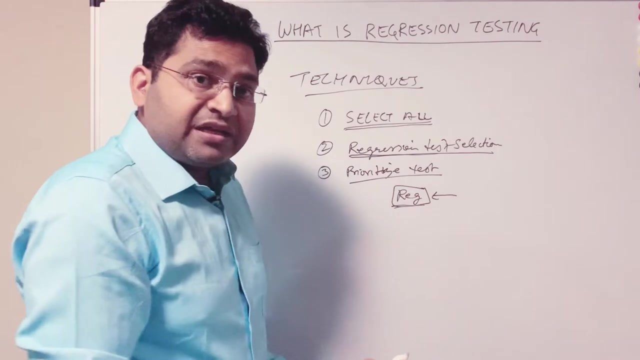 cases of your application. Okay. So when say, for example, your application is already in production and all the major functionality or the critical functionality that is being used, uh, you know every day. So those test cases will be prioritized and in case of any functional changes, any defect, 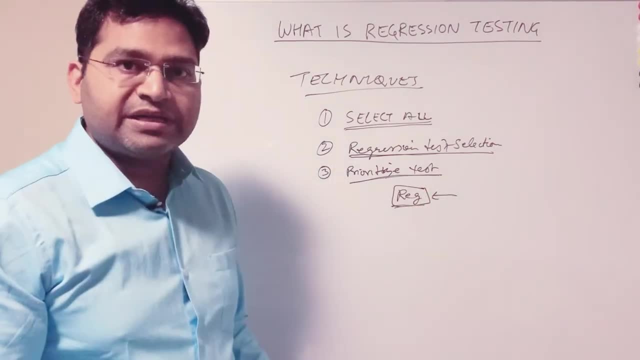 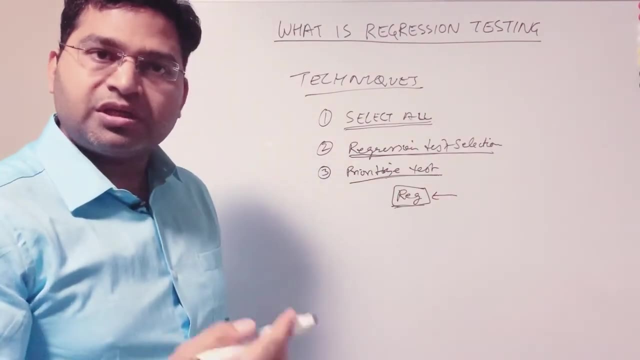 fixes, The prioritized test cases will be executed as part of the regression testing right? So these are some of the techniques that you'll utilize to do the regression testing. Now, when we talk about you, know how you can select the regression test cases. 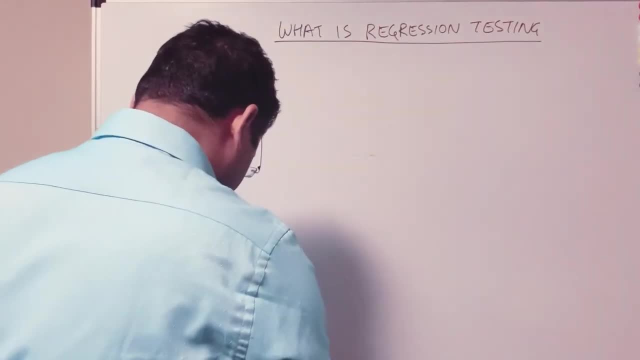 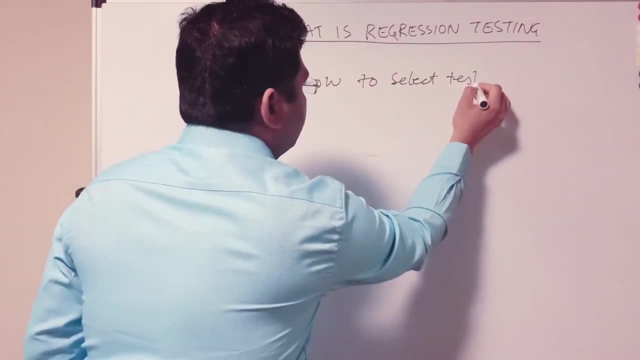 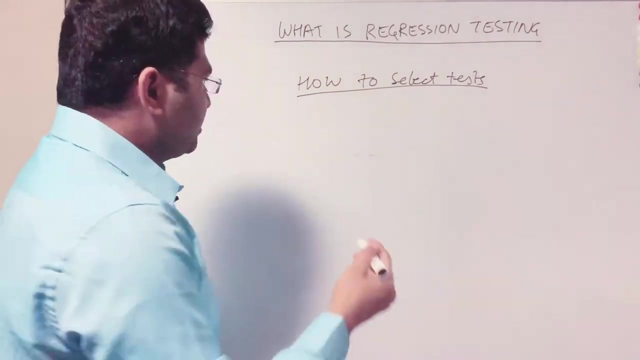 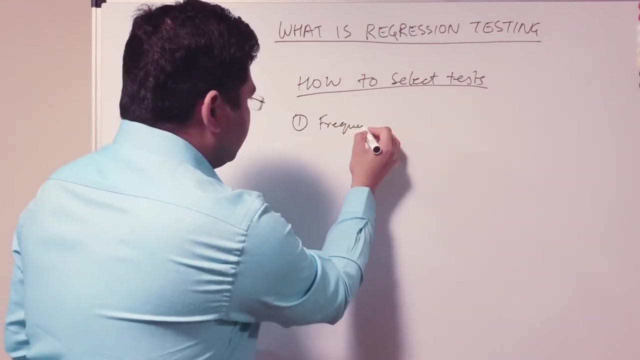 So let me explain how part of the regression testing as well. So how to select, how to select tests. All right Now, So to understand how to select regression test cases, what you need to uh understand is basically uh say, for example, first thing is to um say frequently used functionalities. 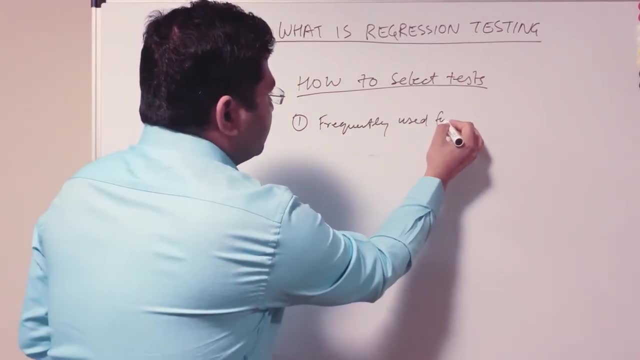 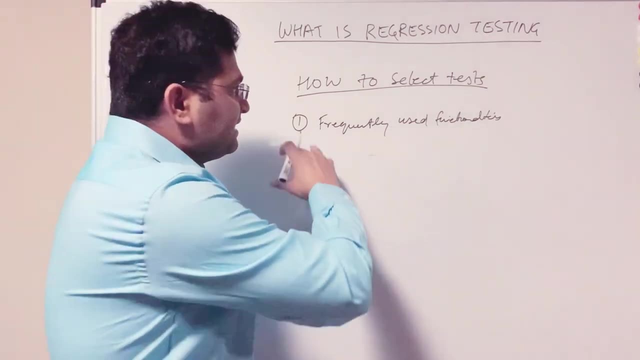 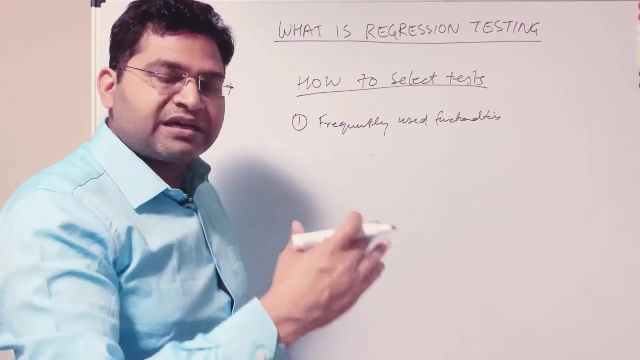 right, So frequently used functionalities. So this is one of the criteria that you can utilize to identify your regression test cases. So in the project when you're working, you will have the prioritized- Okay, Um, uh, you know- functionalities or the critical functionalities that are used very widely. 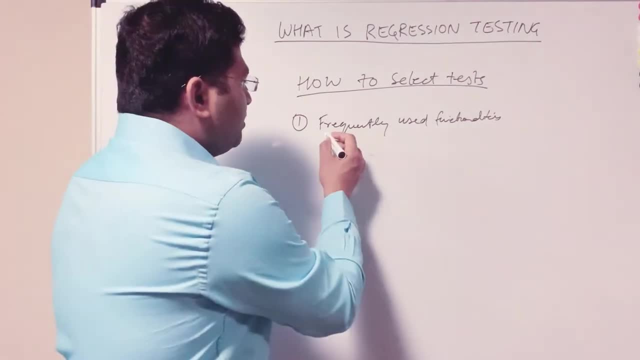 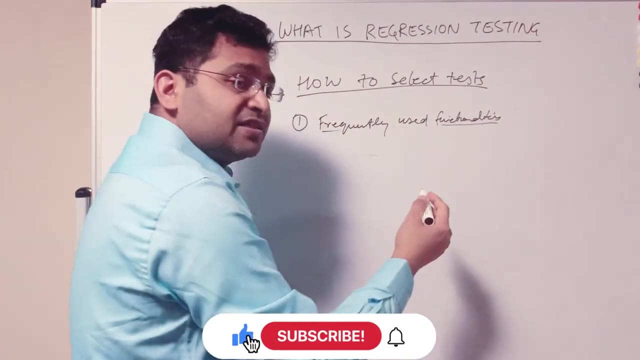 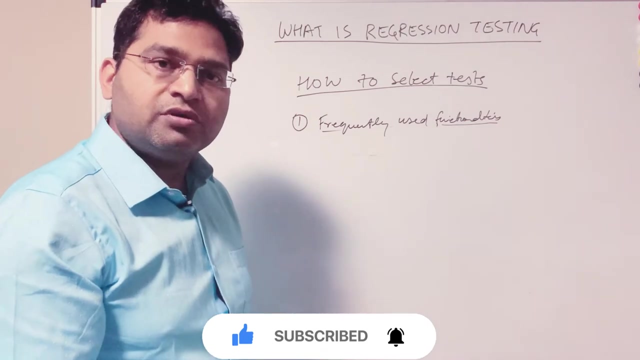 by the app, by the end user or by the customer, then if those are the used functionalities or the frequently used functionalities, then those functionalities or any test cases related to this, that functionality will have the test cases. Those test cases will be critical for your regression testing and you need to pull out. 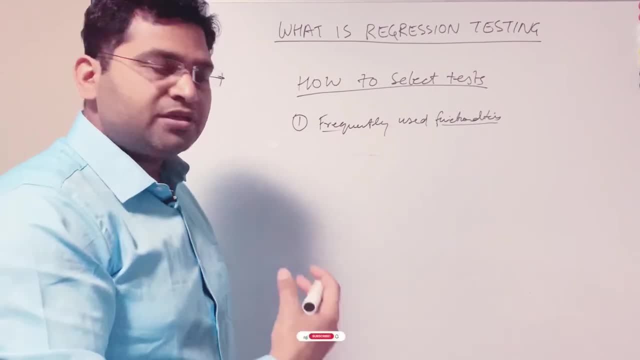 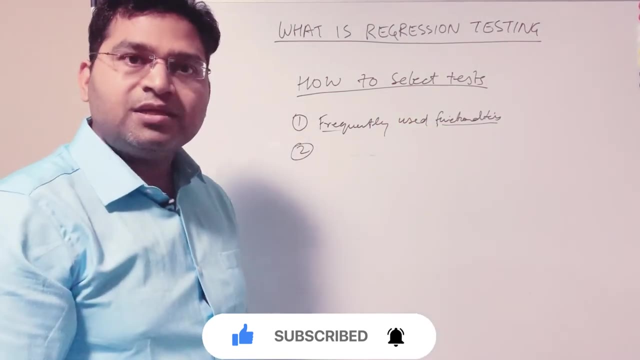 those test cases and have those into your regression test suite. So this is the first you know approach that you can use to select the test cases. So, critical functionality: pull out the test cases for those critical functionality uh in your application. 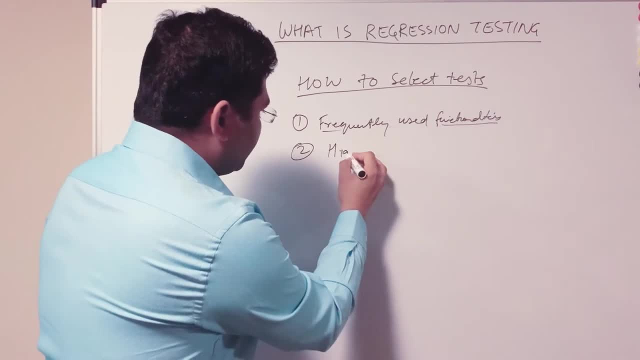 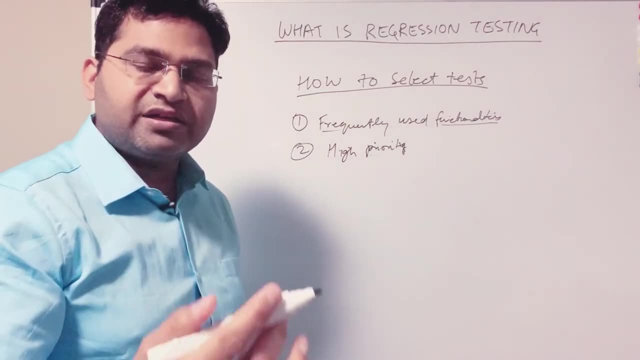 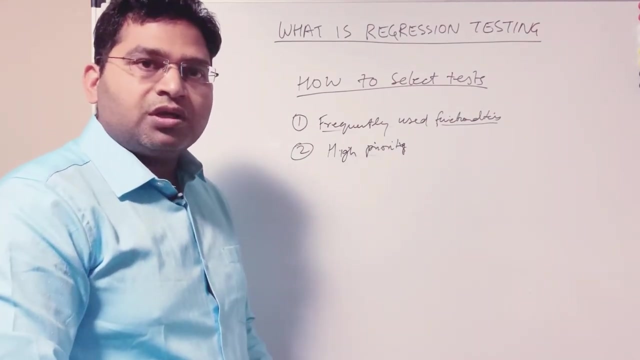 The second is basically high priority, So based on uh, the priority, so high priority. So if you have uh, you know the test cases, you will have the priority assigned to those test cases. So second approach is uh in case of any changes or new functionality or new uh implementations. 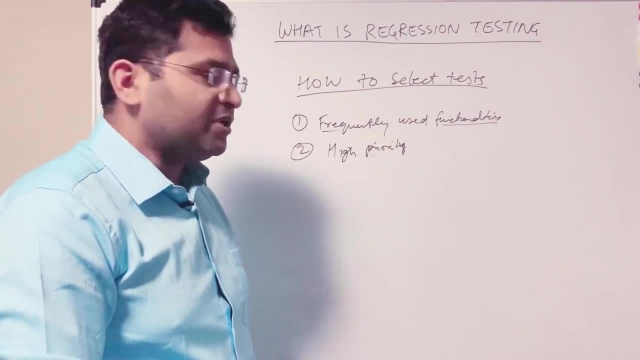 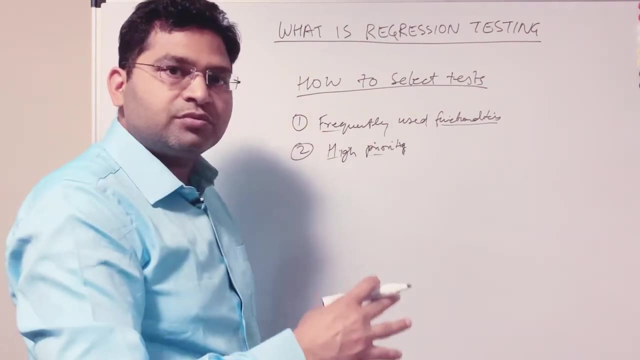 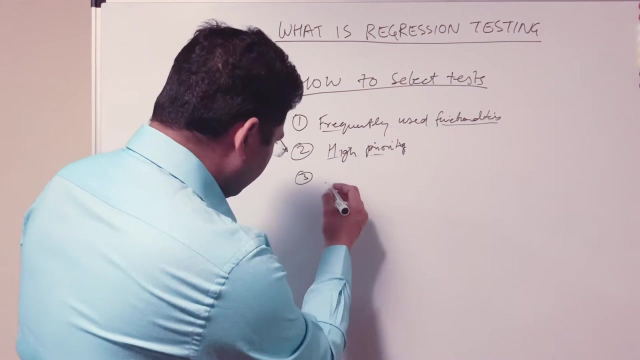 uh, new feature being added into the application. you pick all the high priority test cases that you already have and you allocate those as a regression test suite and execute those. Uh, the third criteria could be your say, for example, integration test cases. right, 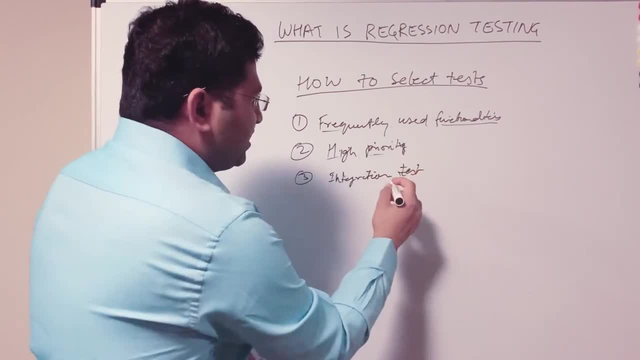 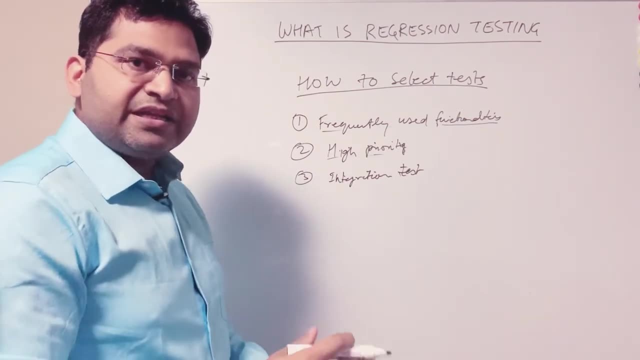 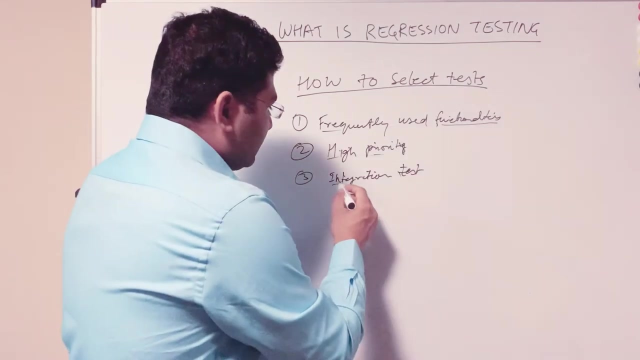 So integration test cases are- uh, you know another very important test cases because when you have the application it will be integrated with other N number applications and if there are any updates in the application, you want to ensure that all the integration points are working as expected. so this is. 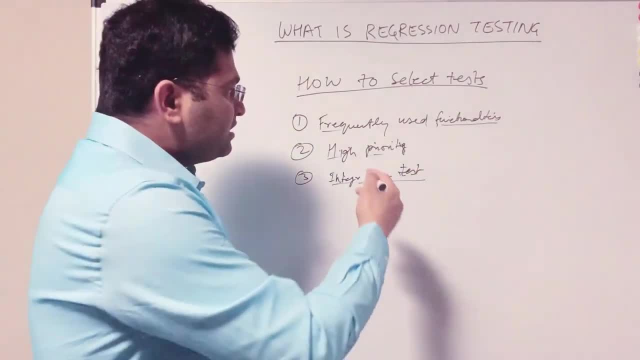 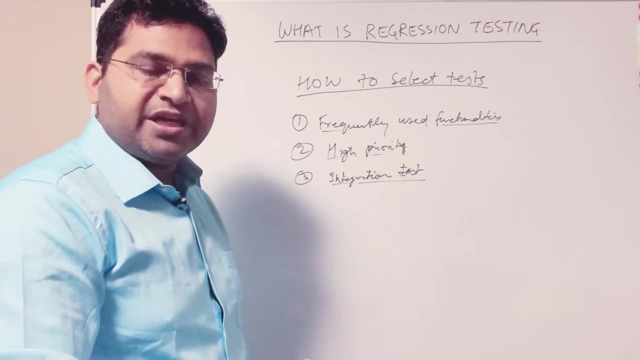 another criteria to pull out the regression test cases. so these are some of the key criterias that you can utilize to pull the regression test cases and create your regression test suite and make it ready to be executed when, whenever there is a you know defect fix or new functionality added right, the 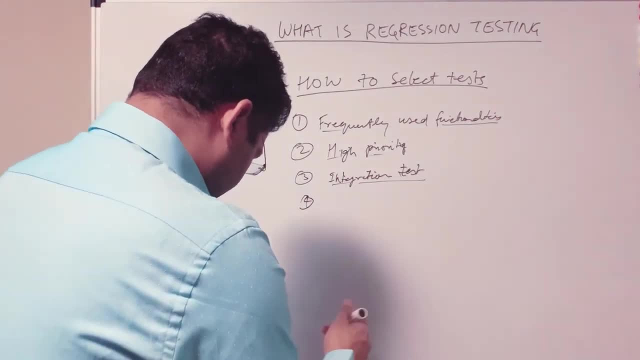 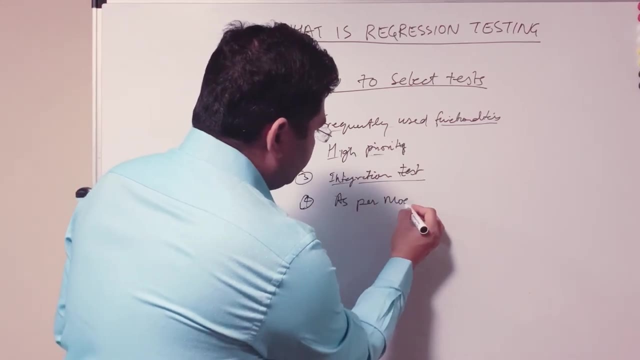 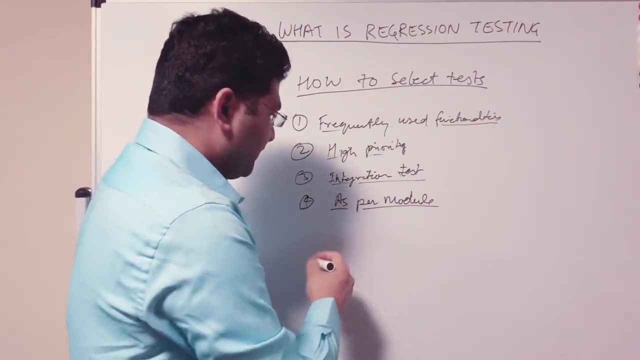 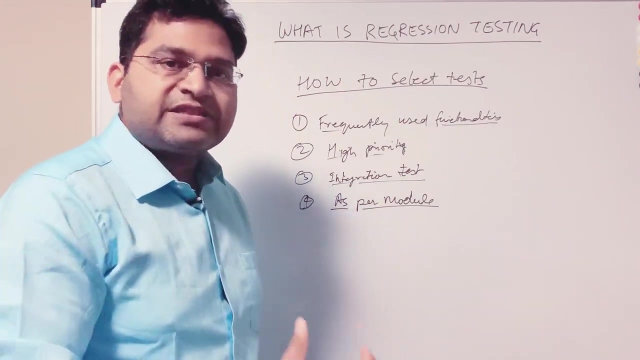 third, the. the next one could be: you know, say, for example, select test cases as per module, so as per module, so when you, when you do this, so when you select as per module, then in that case same example, login functionality, so in that case you analyze what fix has been done in the software application and based on